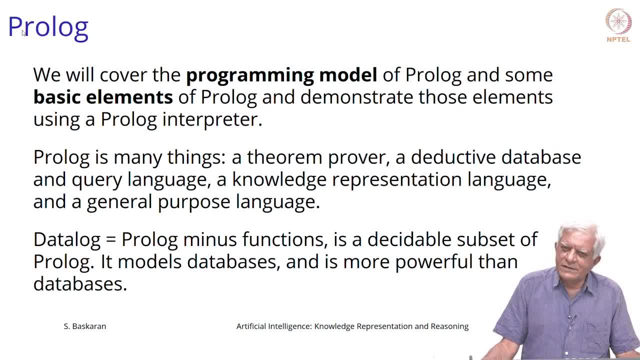 the perspective as a theorem prover. we have talked about deductive retrieval earlier, so we can think of it as a deductive database and a query language for querying that database. We have already started by saying that it is a knowledge representation language and 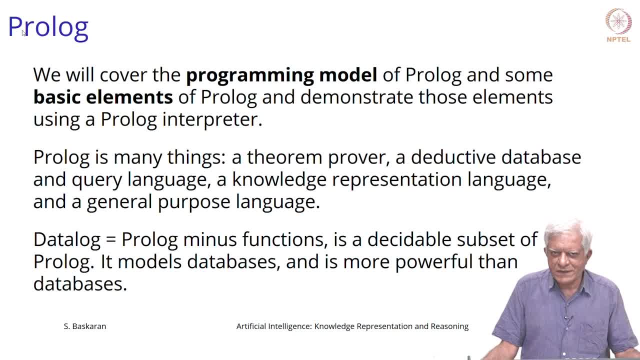 now we are also saying that it is a general purpose language, that it is a Turing complete language. whatever you can do in any other language, you can do with prologue. essentially, There is a subset of prologue called datalog, which is prologue without the function. 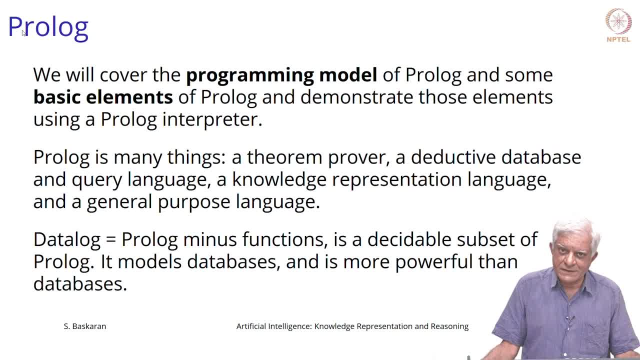 So remember that a logic language is made up of predicate symbols, function symbols and constant symbols. datalog does not use function symbols, and that makes it much more efficient. In applications where you do not need function symbols, datalog would be a good option. 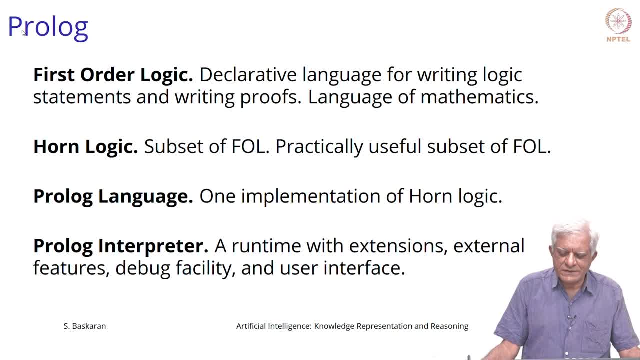 So just a recap. first order logic is a declarative language for writing logic statements and writing proofs. essentially, it is like a language of mathematics. Horned logic or horned clause logic is a subset of first order logic and it is been adopted because of the fact that theorem proving is efficient in that. 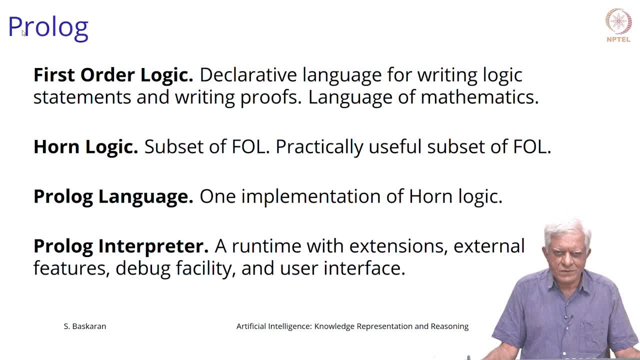 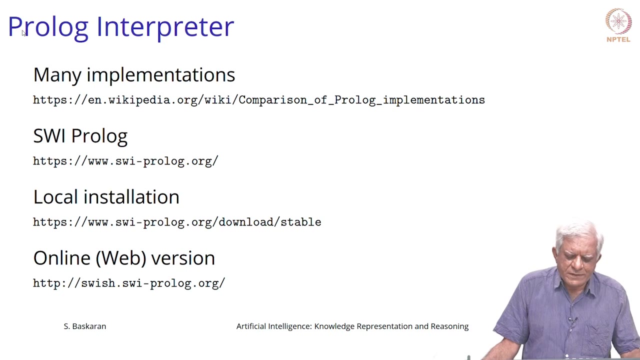 Prologue language is one implementation of horned clause logic and a prologue interpreter would have things like runtime extensions, external features, debug facilities, software or interface to write programs and so on. like any other programming language, You can look at some of these implementations of prologue to practice what we are talking. 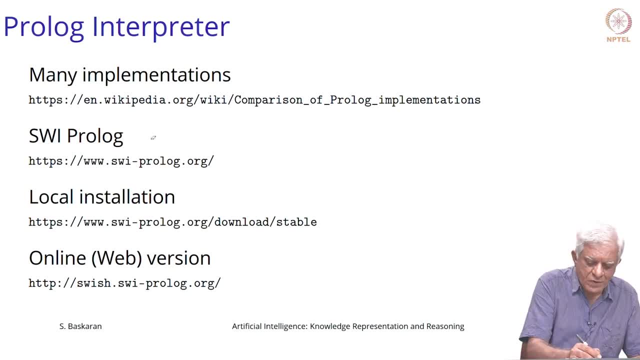 about S2I. SWI prologue is a is a commonly used implementation and you can download it easily from this website and install it and test it out If you are interested in a, if you do not want to download it and if you want to use. 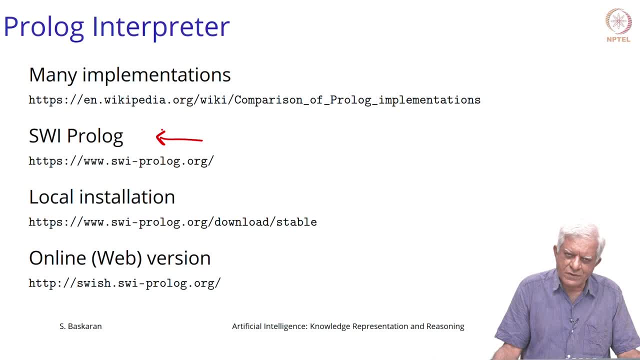 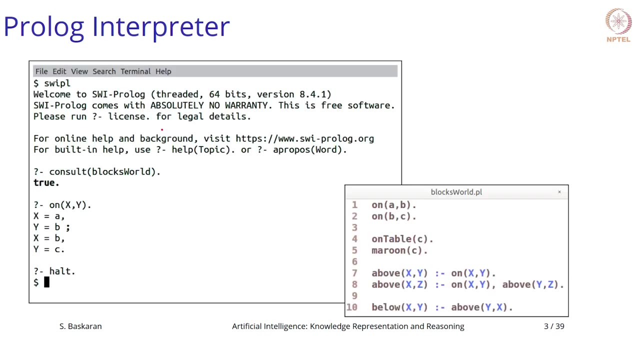 an online version, then you can try this swish SWI prologue which is available, which can be executed online, and you may find other implementations of the language. essentially, Thank you, Thank you. So if you were to run SWI prologue as shown here, you will get a welcome message and then 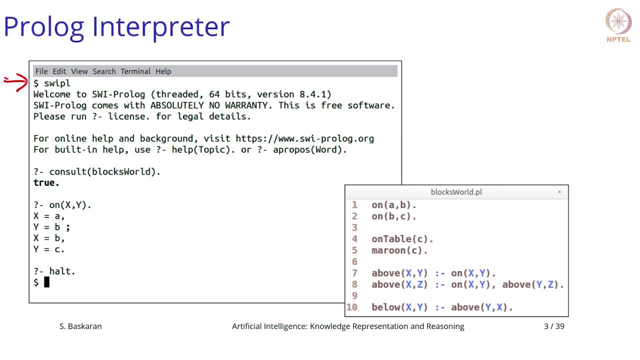 you can proceed. essentially Now, what SWI prologue gives you is interface to ask queries of whatever is a knowledge base. So if you want to enter the knowledge base, the knowledge base can be entered by this command called consult, a file called blocks world. 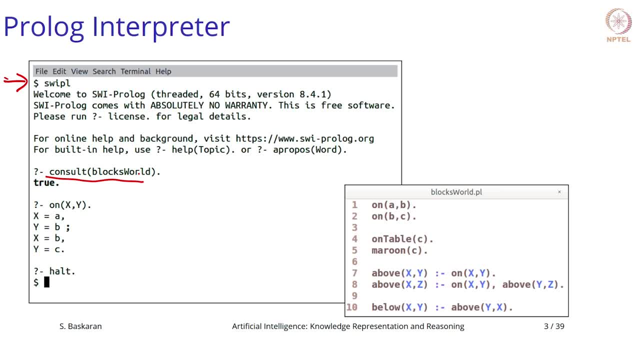 What does blocks world look like? You can see on the bottom right of the screen that, as you can see, it is. it is a. it is a prologue program and we have already introduced a little bit of the syntax. we have some statements. 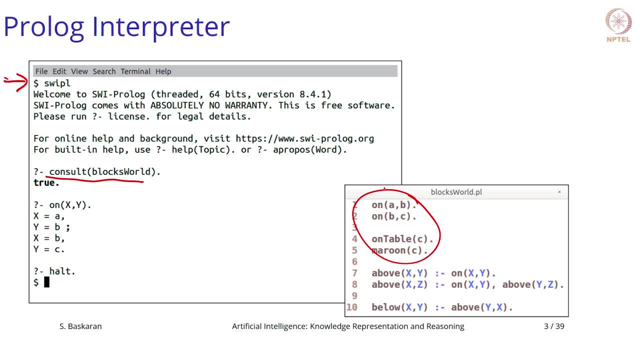 which can be called as facts: A is on table, A is on B, B is on C, C is on table and C is maroon. Then we have rules for defining the above relation. We have the on relation. we want to define the above relation, which is a recursive relation. 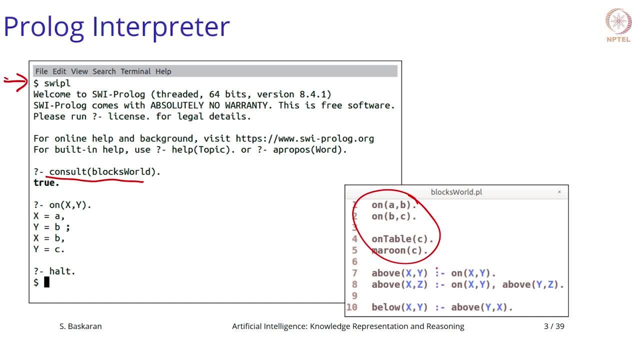 We have already seen flavors of this. This says that X is above Y. if one option is that if X is on Y, if it is, if it is on Y, then it must be on above. That is the first or the base clause. 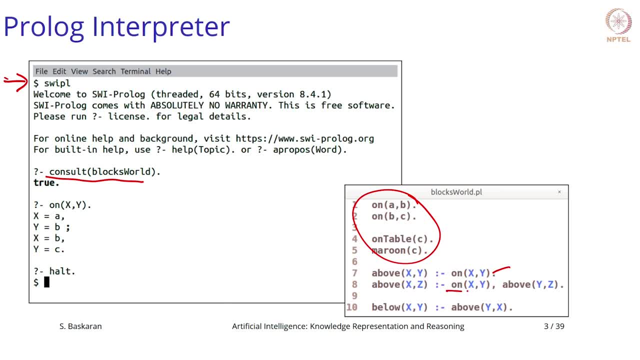 Reversive clause says that X is above Z if X is on Y and Y is above Z. So if you remember the grandfather grandparent relation we had defined earlier or the connected graph relation, it is very similar in flavor to that. 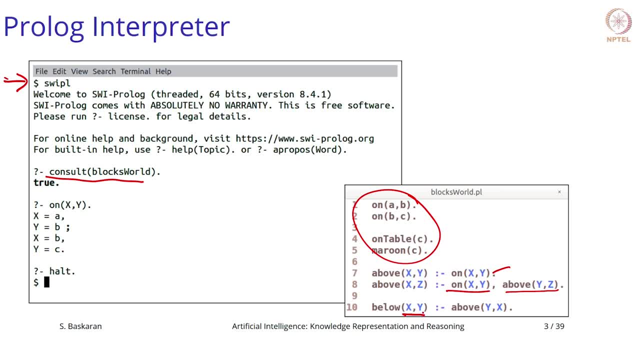 You can also define the inverse relation. You can say that X is below Y if Y is above X. essentially So, when you say consult blocks world prologue will S to Y, SWA plus X, SWA prologue will load your program and it will be ready to answer your queries. 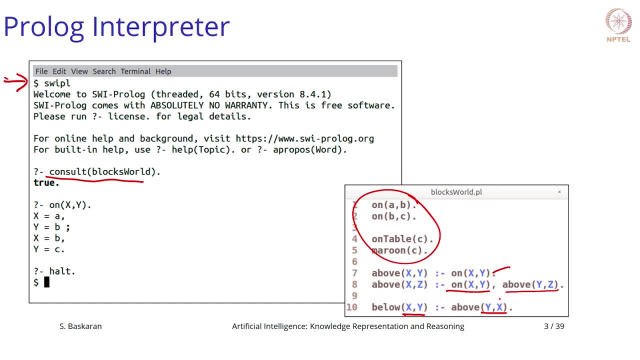 So when you type in something, it is treated as a query. So here you have typed in a query which says: is there some X which is on Y is where Y is also something, and prologue will, in this version, will, give you all the answers. 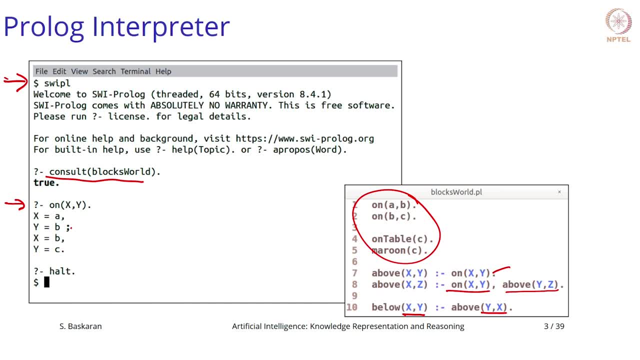 It will say: X is equal to A, Y is equal to B. That is one answer delimited by a semicolon. Then we have a problem. We have a problem, We have a problem. Then the second answer: X is equal to B and Y is equal to C. essentially, 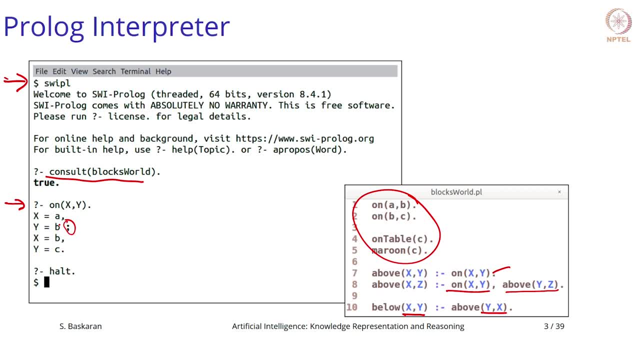 So you can see that both these answers are true. for on the query on, because we have said that A is on B and B is on C, essentially. Now some versions of prologue will give you all the answers. will try to give you all. 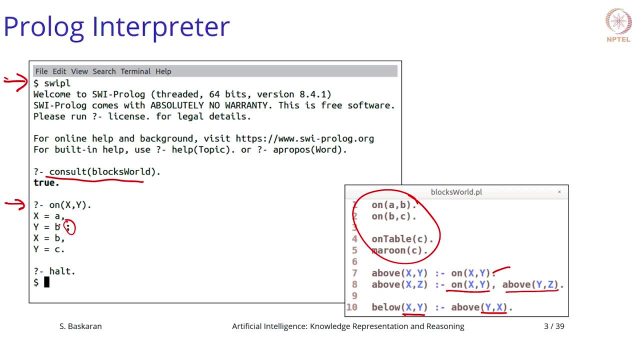 the answers. Some version will will give you one answer and you will have to press the carriage return to get the next answer. Anyway, that is a matter of implementation. You can give a command called hold, Which means I am done with this session, and it will terminate the session. 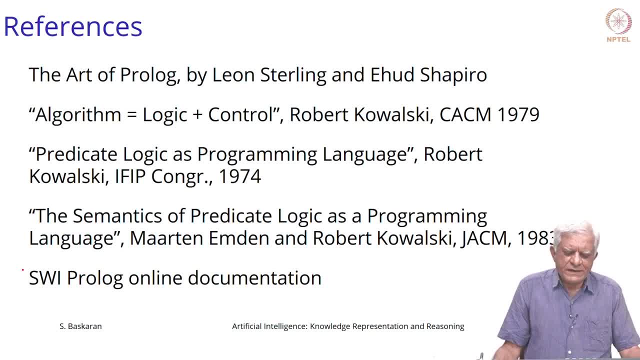 There is a very nice book on prologue. it is called The Art of Prologue, by Sterling and Shapiro. I use it in courses where I teach logic programming And if you can get your hands on it, it it is. it is really a good book. 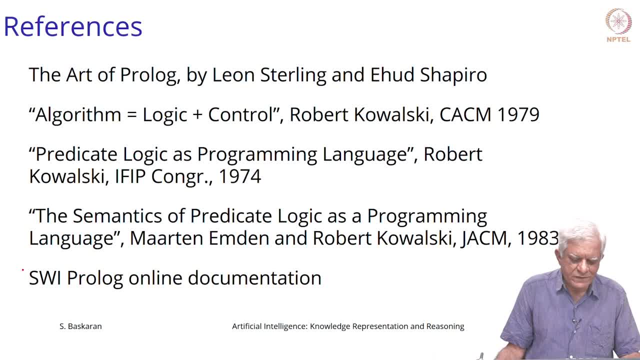 Then there is the original paper by Robert Kowalski from 1979, which is titled: Algorithm is equal to logic plus control. We have already spoken about that And there are some couple of more references that you can see to which tell you more. 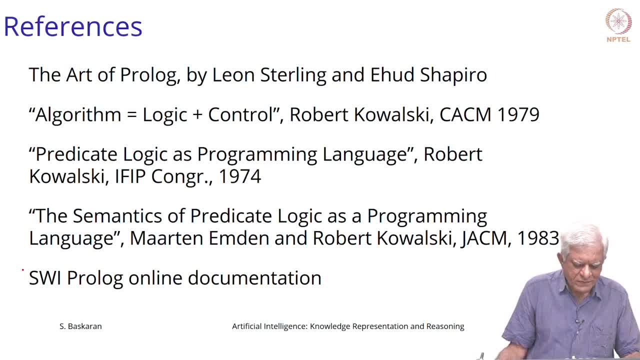 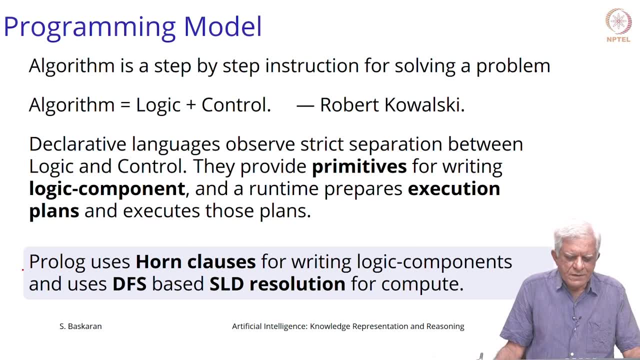 about prologue. You can also look at the documentation of SWI prologue. So the programming model for prologue, that algorithm is equal to logic plus control. Now our notion of of a algorithm or a program is that it is a step by step instruction for 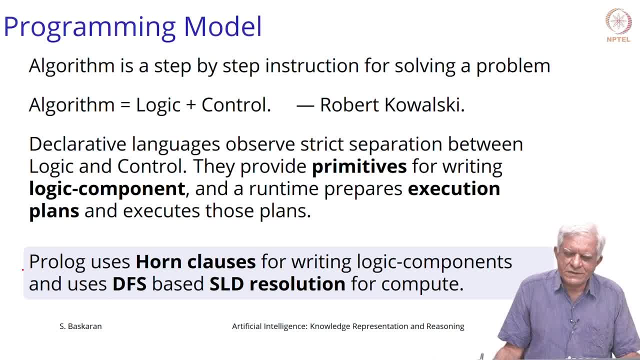 solving a problem Which is closer to our notion of imperative programming. a programming language like C, for example, Would say: X is equal to 13,, Y is equal to 41,, Z is equal to X plus Y minus 3.. 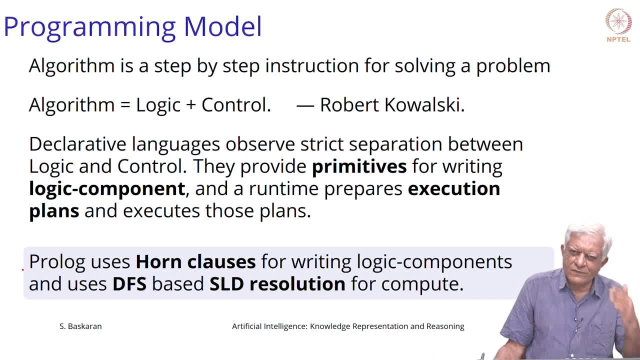 So you can write statements one by one And that is how the flow of control is part of the code In. we have declared, we have- we have kind of discussed this earlier- That in logic, In logic programming, which is a declarative style of programming, we want to separate. 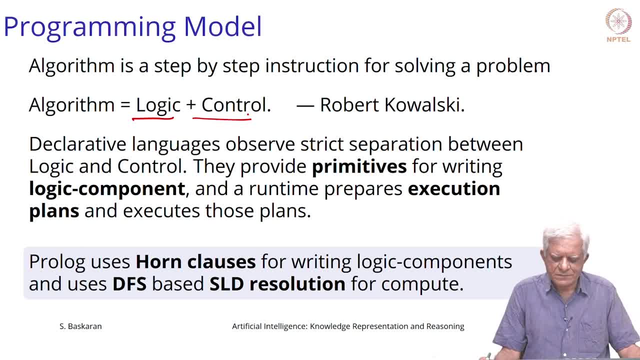 the two parts of the algorithm, the logic and the control. So they provide us primitives for writing the logic components, like F O L, for example, And a runtime prepares an execution plan and execute. So the execution is not in our hands. there is a interpreter or an inference engine which 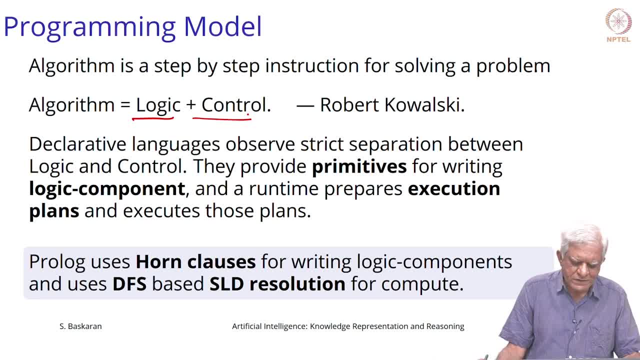 does it for you Now. prologue, as we have already said, uses the horn clause, subset of logic Because it is more efficient and it does, as we saw in the case of backward chaining. it does depth first, search over the tree, essentially, which corresponds to SLD resolution for horn. 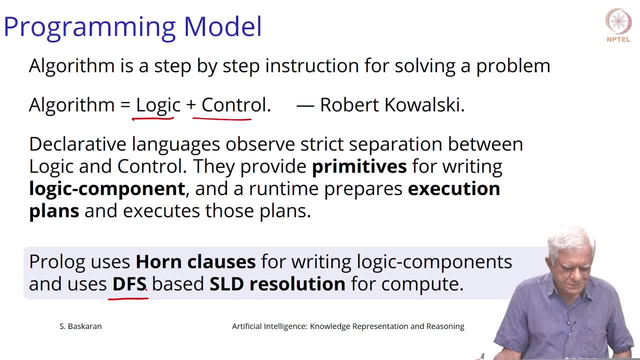 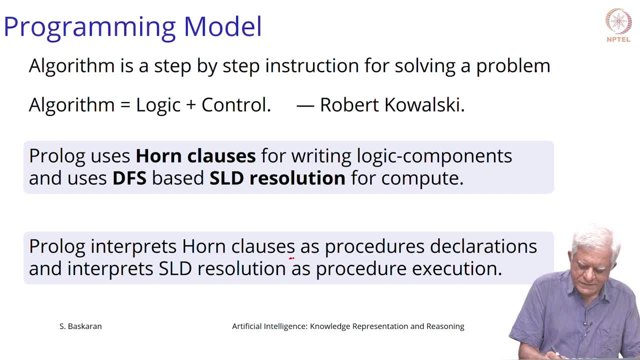 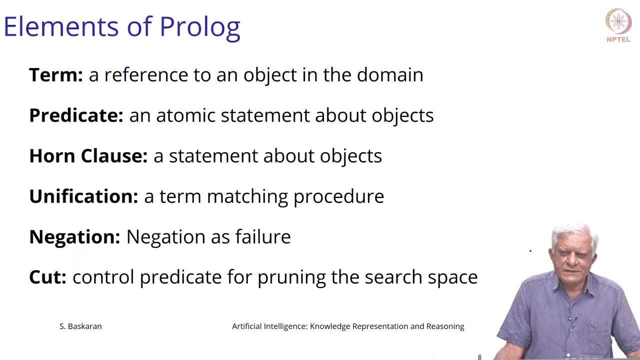 clauses. Remember, we will define horn clauses again as we go along. Prologue interprets horn clauses as procedures, as procedures declarations, and interprets SLD resolution And as procedural execution. I hope we will get a flavor of this as we go along. 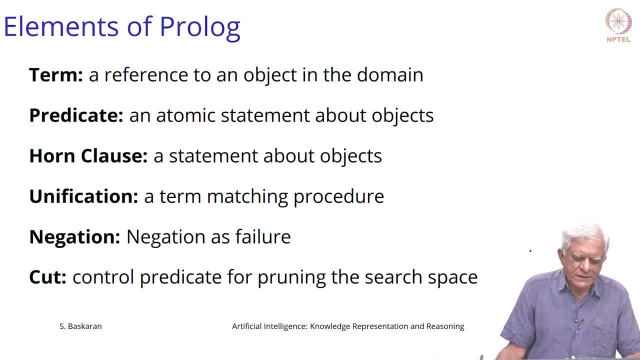 Some terminology, a term in logic and in prologue is a reference to an object in the domain. So we have defined the family of terms earlier. A predicate is an atomic statement about those objects. it is a relation on of some on those. 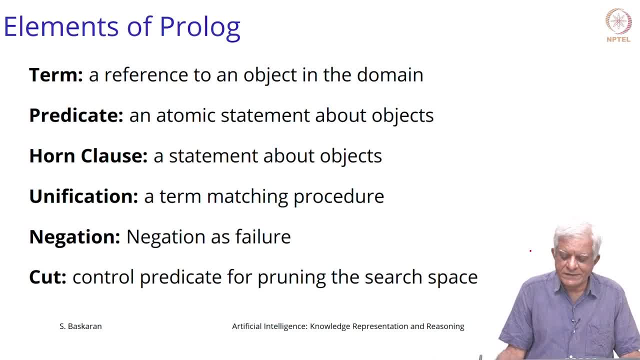 objects. A horn clause is a sentence, a statement about objects. It includes atomic predicates and logical connectives connecting them together. Unification is a process that we use for matching two terms. Negation, as we will see in the near future, will be treated as negation, as failure in 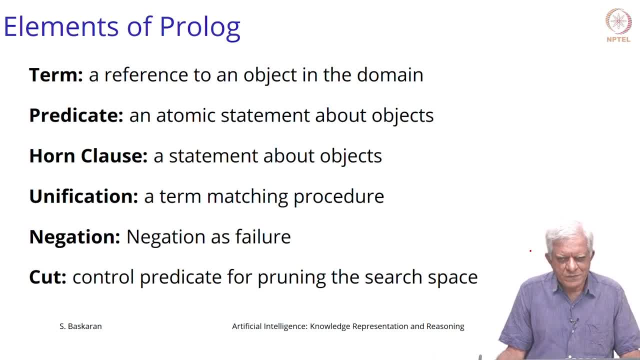 prologue, which means that if you cannot show that something is true, Then you assume that it is false. and that is how prologue treats negation. So it is a closed world assumption. it says that if I cannot show that it is true, then 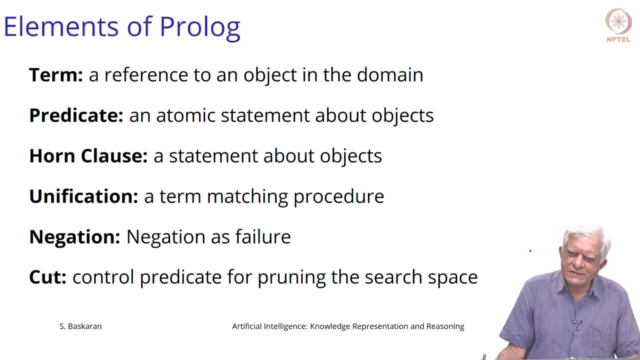 it must be false. We will look at a procedural tool called cut, which is used to make programs more efficient because essentially prologue is searching over a knowledge base, And to avoid some repetitive searches. in many situations prologue interpreters come with. 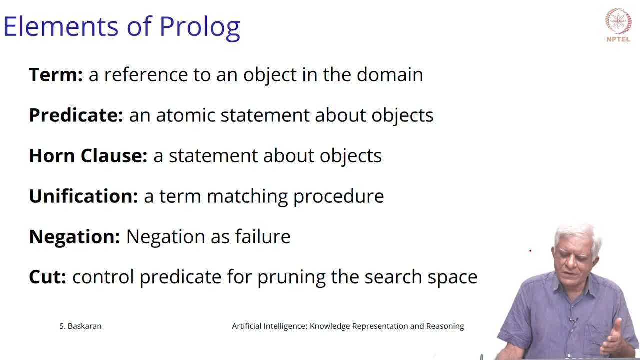 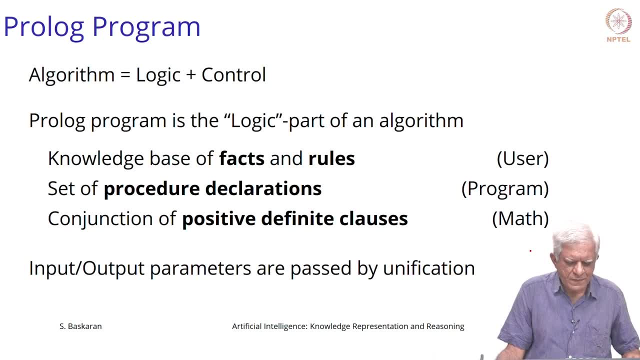 this feature, which is an extra logical feature in some sense, called cut. essentially We will look at that also later. So an algorithm is logic plus control. The prologue program is a logic part of the program. From the user's perspective it is a knowledge base of facts and rules, essentially, 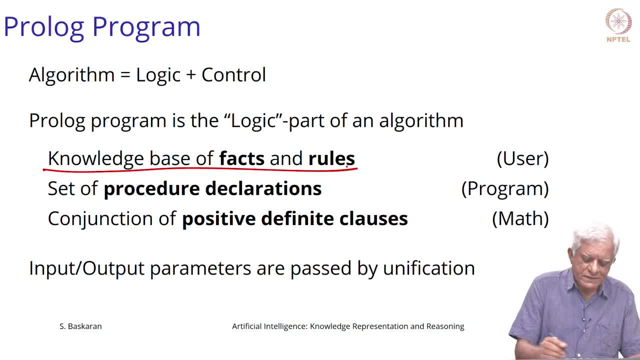 Okay, Okay, From a programmer's perspective, it is a set of procedure declarations. From a maths or a logical perspective, it is a conjunction of a set of positive, definite clauses. The input and output in all these procedure calls is done by unification, and that is.